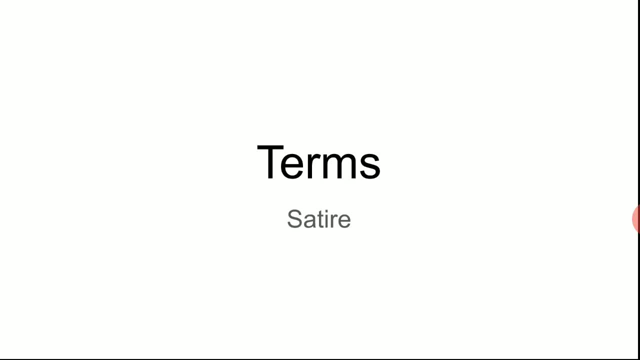 can say It makes the presentation of the work more interesting And its effect more artistic, more effective, and makes it something special from the ordinary speech. By the way, that was the definition. that was the discussion. general discussion about the terms. 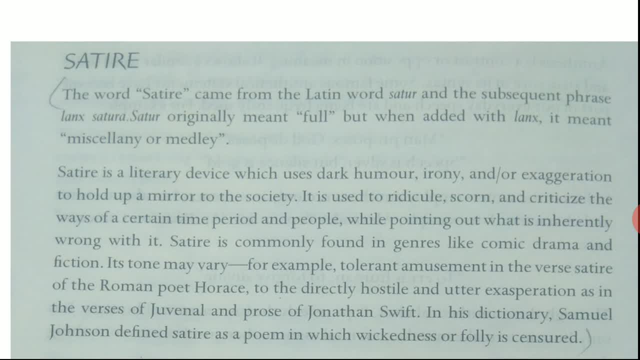 We come to our today's term, which is satire. So it says that satire comes from the Latin word satire. Satire is the word associated with satire, who is the god of wiles, But etymologically, satire means full of medley, full of different types of things. It is a collection of things. 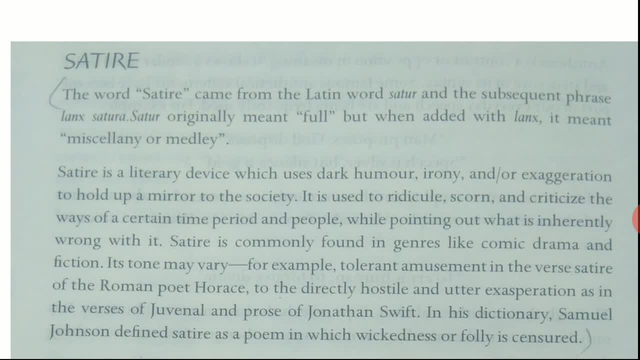 which generally do not go together. We can say: rang birangi tadak bharak jaisi posaag jaisi ki ek joker peinta hai. That type of meaning is in satire, So obviously it makes something funny. 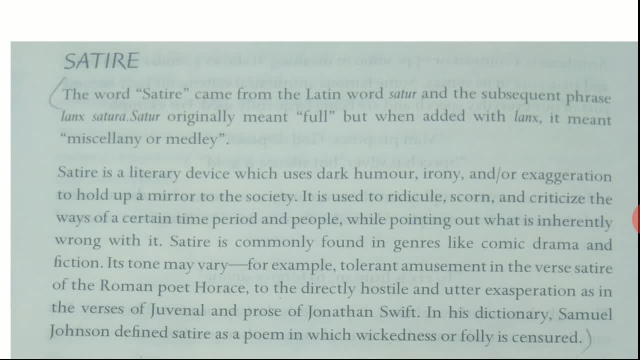 So as a literary device, it uses humor, irony or exaggeration to hold up a mirror to the society. It shows the, it makes fun of a person or an idea, or a custom or a situation. But the real aim of that joke, the real aim of that funny description, humorous description, is: 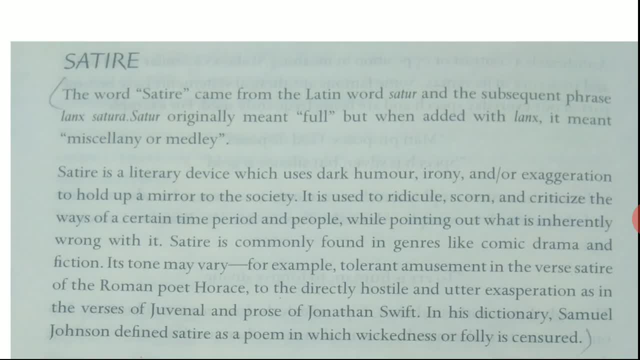 not only to laugh at but to make people laugh. laugh at but to point it out for correction, so that that folly, that malpractice, that defect in character, that vice in character of a person can be brought upward, can be introduced, can be actually, can be explained and the society or that person becomes aware of that thing and he can do. 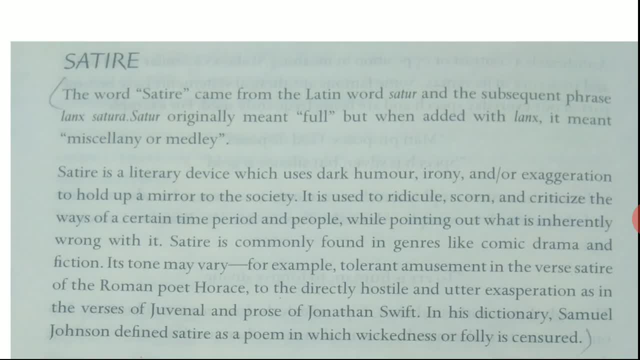 the necessary correction. that is the real purpose of satire. so satire is used to ridicule, ridicule, scorn and criticize the ways of a certain time period and people that in society. it may ridicule the society, any social practice, pointing out what is inherently wrong with it. its aim is to point: 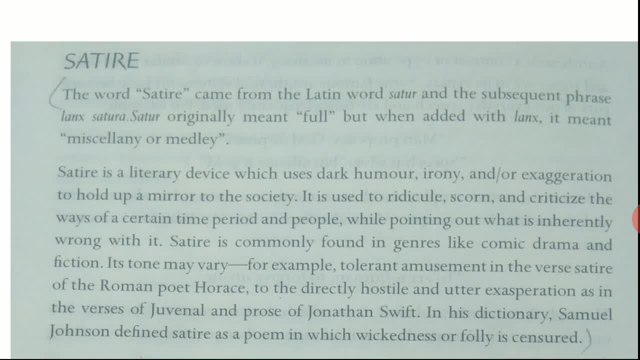 out that defect. satire is commonly found in zants like comic drama and fiction, though it may be in words. also, its tone may vary, for example tolerant amusement in the worst satire of the roman poet horace. that brings us to a type of satire, horatian satire, to the 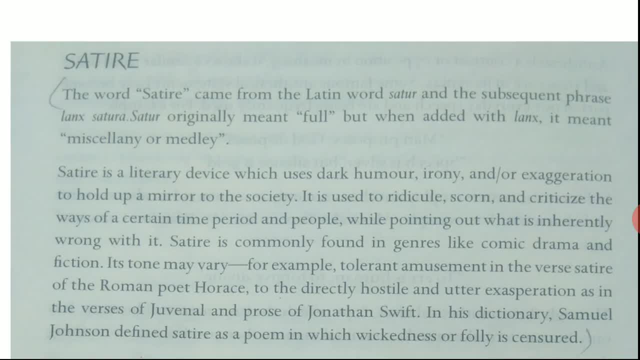 directly hostile and utter exasperation, as in the verses of juvenil and the prose of jonathan swift. that brings us to another type of satire that is jovial. in his dictionary, samuel johnson defined satire as a poem in which wickedness or folly is censored. 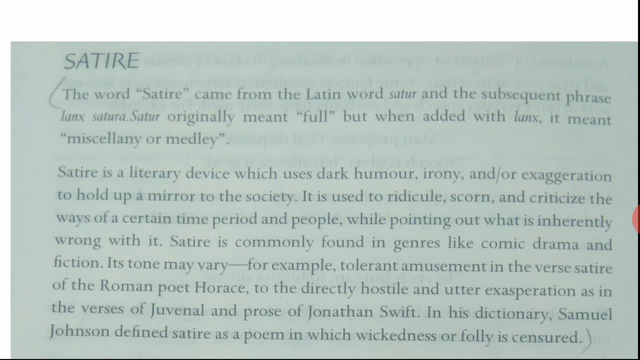 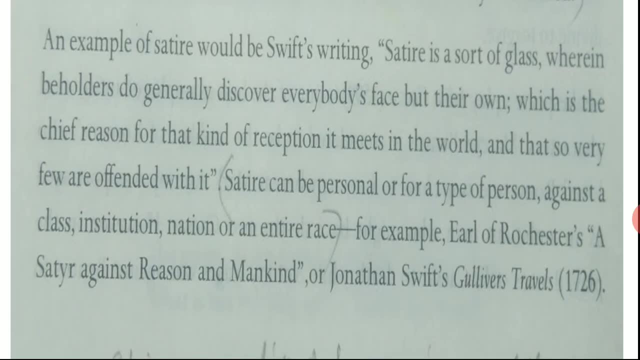 an example of satire would be swift's writing. swift has written so many satires, especially the gulliver's travels, if you remember. he says that satire is a sort of glass wherein beholders do generally discover everybody's face but their own. when it comes to the follies or drawbacks in character, generally we do not recognize 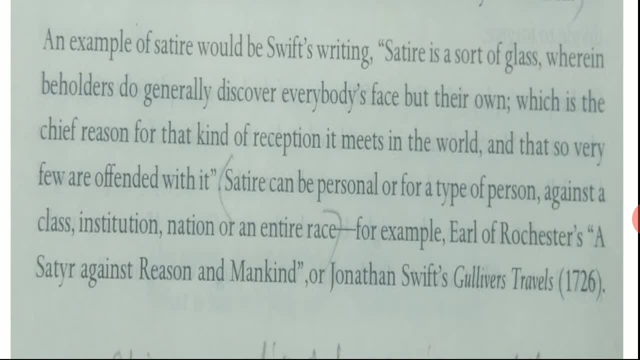 ourselves. but through satire we can get that awareness. that is the effect of a satire, good satire, which is the chief reason for that kind of reception it meets in the world. generally. satires, humorous pieces of writing are always welcome and that so very few are offended with it. 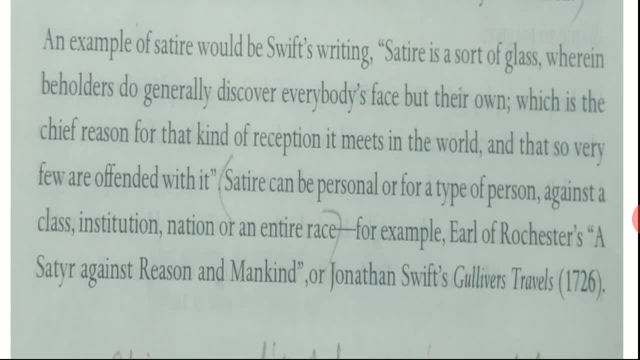 it can be personal or for a type of person, against a class, against an institution, against a nation or against an entire race. it depends upon what is the target area of the satire. jonathan's, gulliver's travels, ben jonson's valpenno satirizes certain types of people and 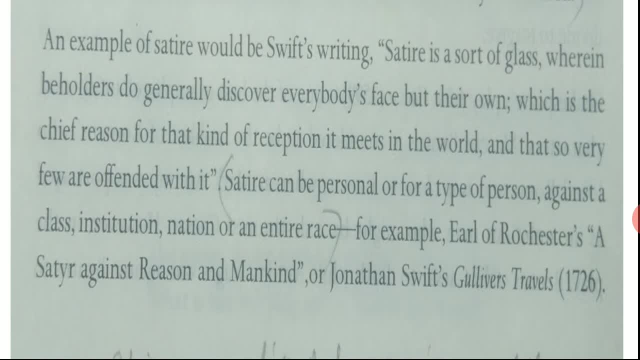 dryden's mcflacknoe represents a kind of pretentious poetaster and satirized especially a rival author of his time. thomas said: well, so it is personal satire. satire may be personal in which a person is targeted. it may be social satire in which the voices or the malpractices in society are discussed. 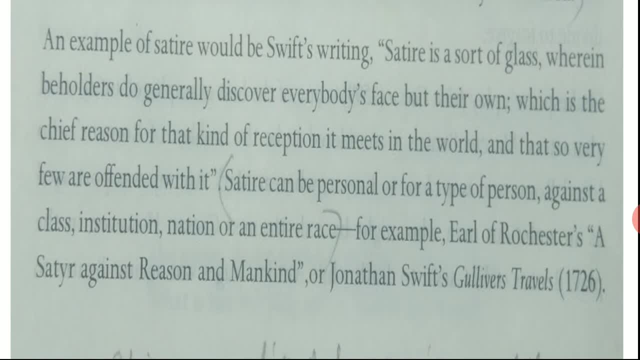 so, to sum up, we can say that it is a piece of writing humorous in nature. it employs humor, irony, exaggeration, and it ridicules, it laughs at something, but the purpose is to expose and criticize people's stupidity or vices for correction. the real aim of satire is improvement through correction. 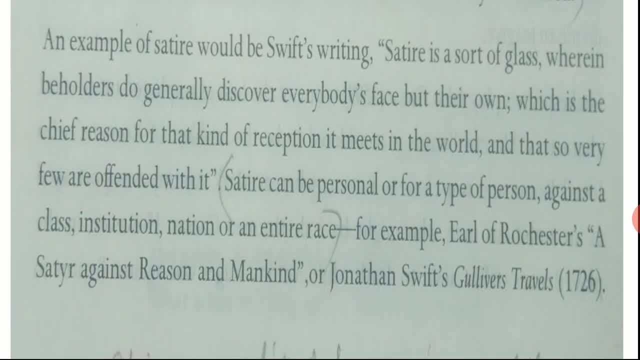 it is an extremely broad category. we can say that it may involve a humorous piece, an ironic piece, an exaggerated piece, or it may have any one of them. we must remember to identify a satire. we can say that a satire makes fun of a person, makes fun of a practice, a situation, an idea or an institution. 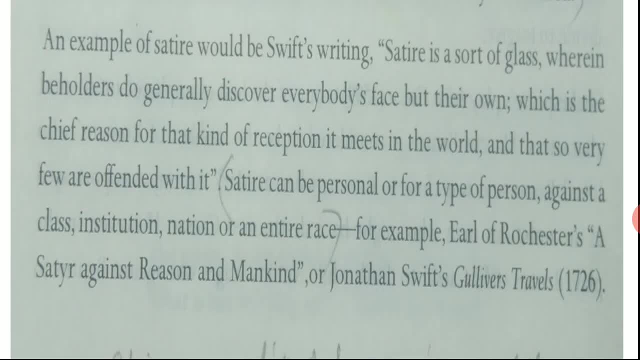 one of these are the target subject of a satire. these things are ridiculed in a satire. but second thing we must remember is that its purpose is not only to entertain or laugh at but to inform about that fault and to make people think, make society aware of that vice, aware of. 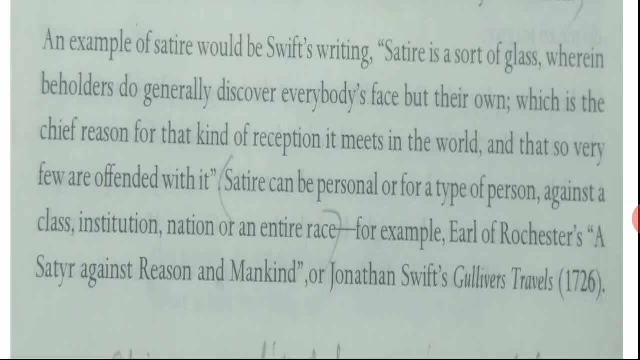 that wrong thing, so that it can identify it and make correction. so correction through humor is the aim of a satire. now there are three types of satires generally: juvenalian satire, manipian satire and horatian satire. juvenalian satire is named after juvenal. it is the strongest type of satire and it attacks a. 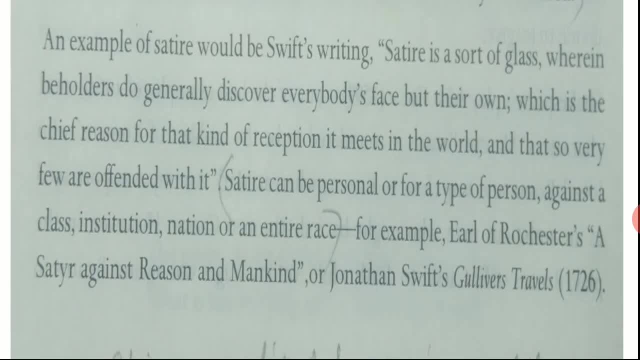 single target in a vicious way. it is very cruel in its treatment of the subject. the most common form of this satire is political satire, which attacks politicians and pundits. so juvenalian satire is personal satire and it attacks ruthlessly. generally these things are not accepted by common readers, but still they serve the purpose. then the manipian satire. this